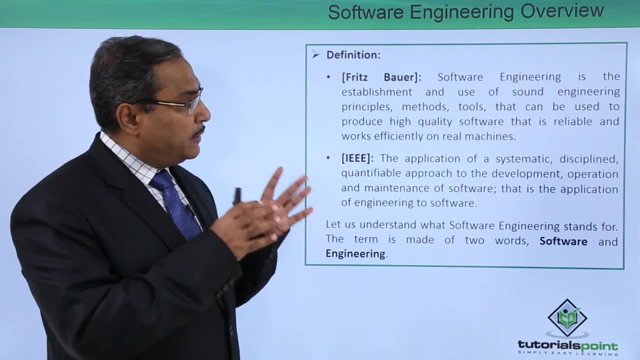 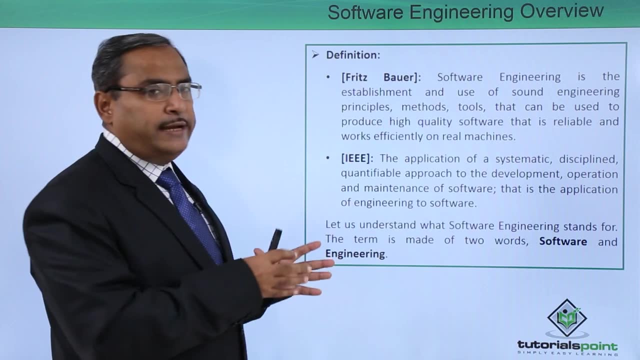 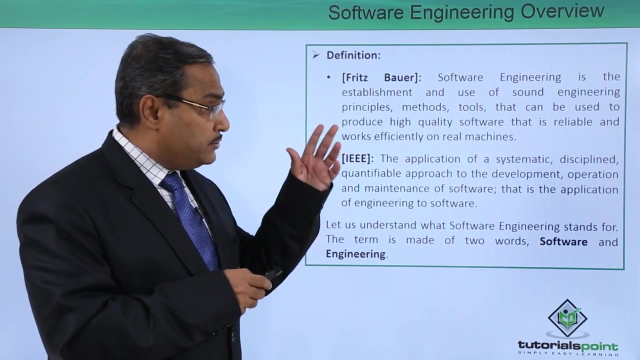 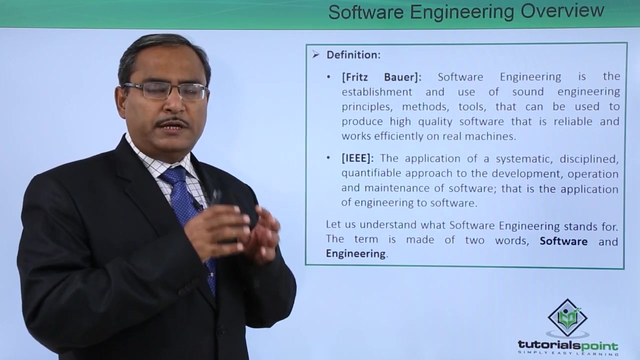 then he has defined the software engineering in this particular format That is, software engineering is the establishment and use of sound engineering principles, methods, tools that can be used to produce high quality software that is reliable and works efficiently on real life. So the software should be reliable, should be meeting with the respective users requirement. 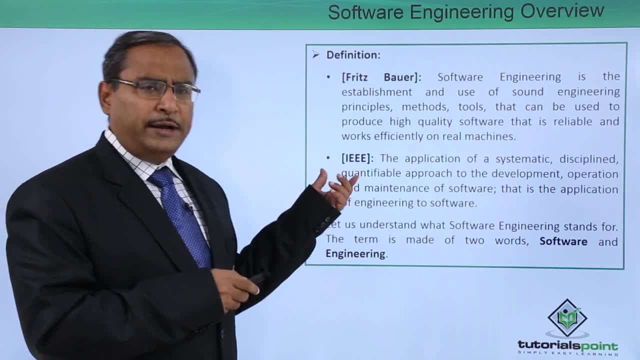 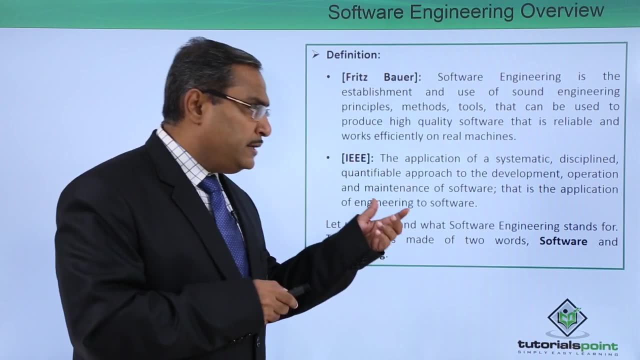 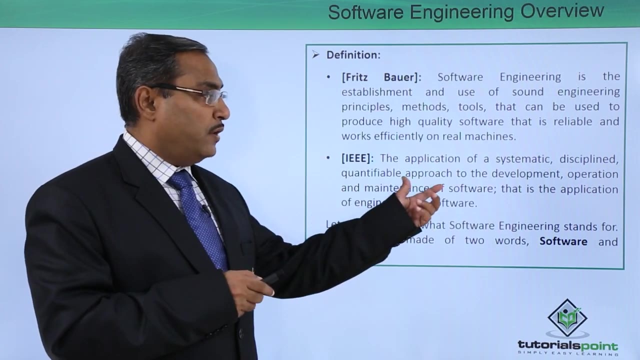 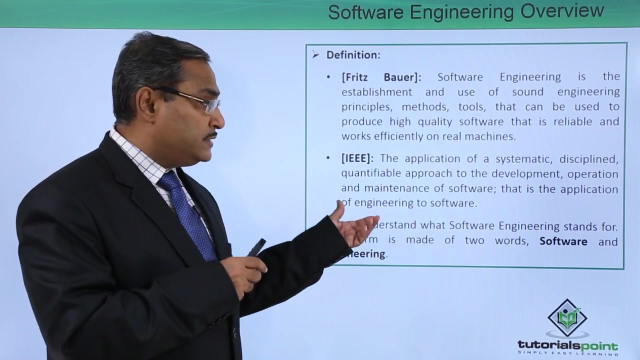 and should run on the real machines, IEEE. they have defined the software engineering in this way: The application of a systematic, disciplined, quantifiable approach to the development, operation and maintenance of software. that is, the application of engineering to the software. That means they have given emphasis more on the overall development process there. 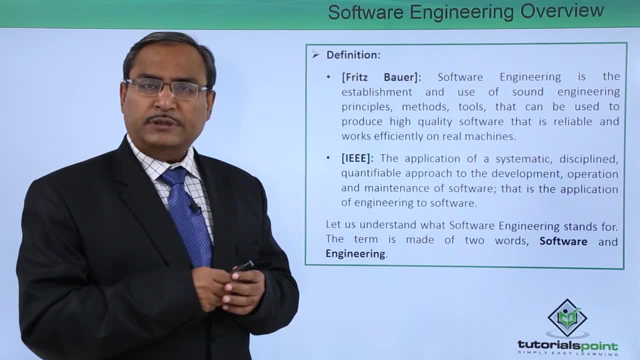 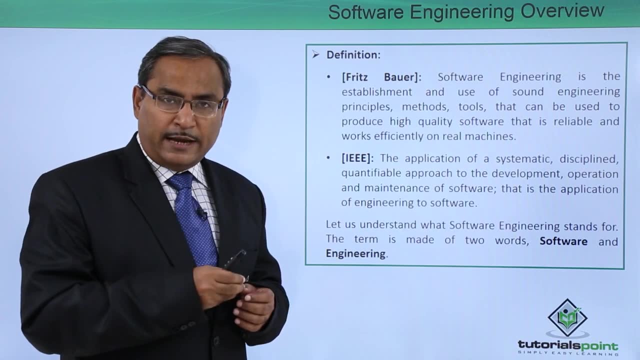 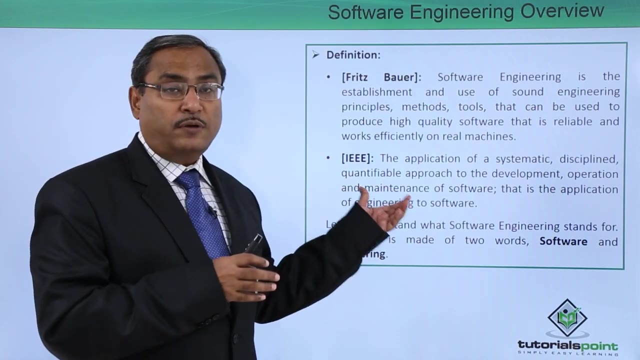 is an operation to be implemented, the maintenance of the software during the upgrading of the software to execute some change request as requested by the client. All those things must be done on this respective software product and this software playback software, and that is why this IEEE, they have given more emphasis on these operations and the maintenance of 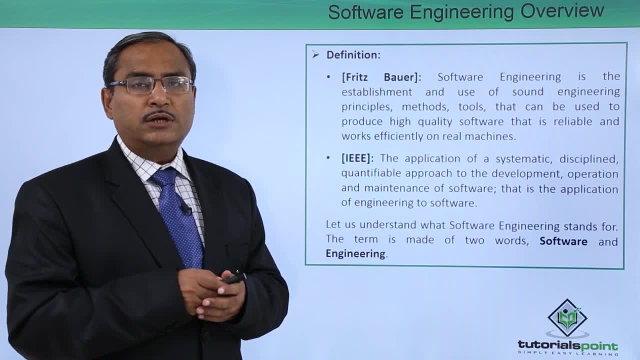 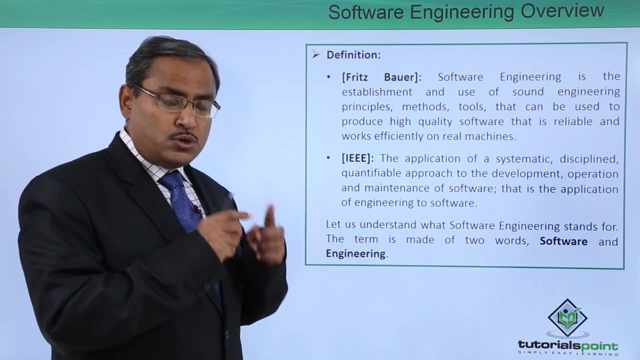 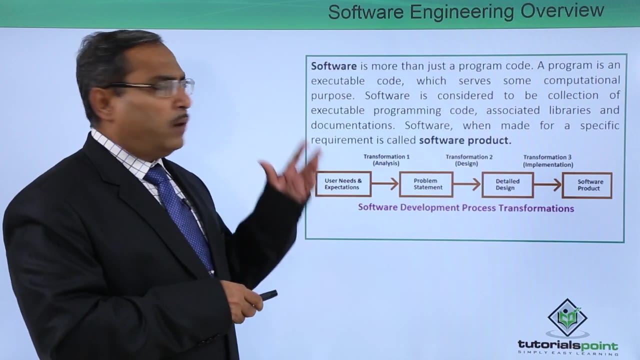 software, and that is application of engineering to the software. Let us understand what software engineering stands for. and here we are having two terminologies: one is the software and other one is the engineering. So let us discuss them one by one. So what is the software? 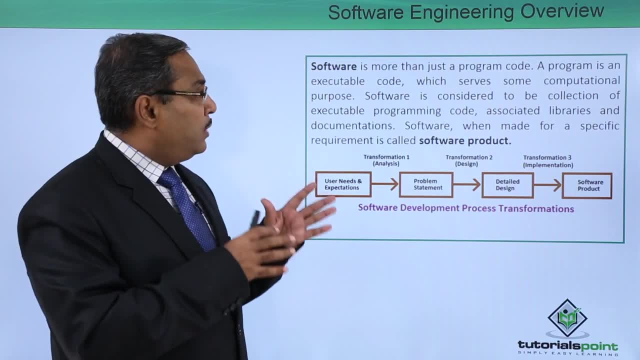 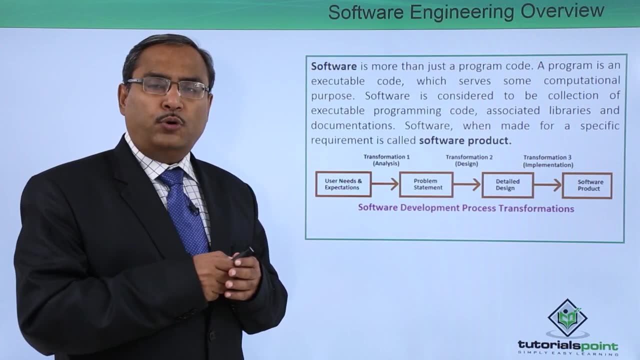 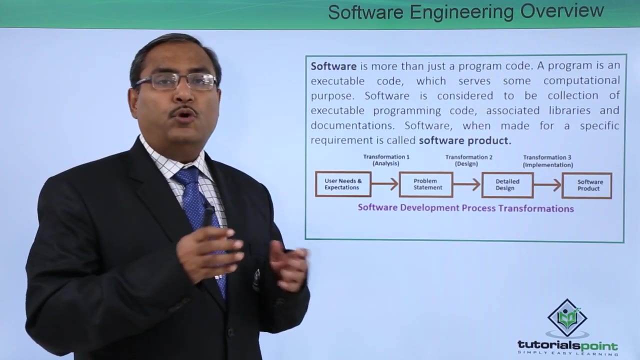 A software is more than just a program code. A program is an executable code which serves some computational purpose. We know that whenever we write any program in some specific language, then obviously it is having some purpose and at the end the program should be executed through the executable. 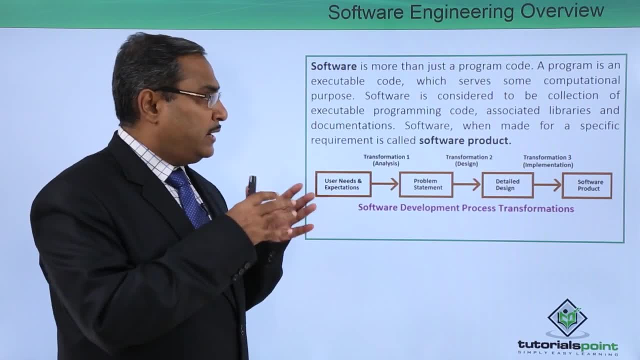 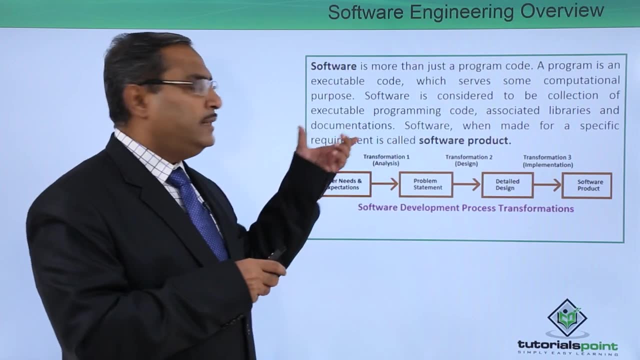 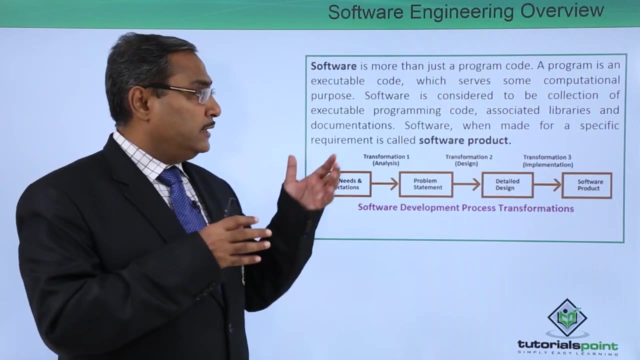 version of the program. A software is considered to be collection of executable, such programming codes, libraries, and then associated libraries, and then documentation and remote and documentation and so on. So what is the software product? So software is nothing. but Whenever a particular software is executing, that means it is taking help of multiple executable.